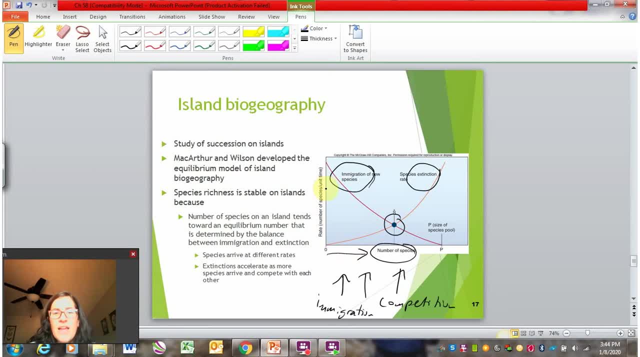 somewhere around here. For a different island, that balance point might be different. So we're not saying that islands always have the same number of species. For a different island, that number might be over here instead, based on different features of the island. Okay. 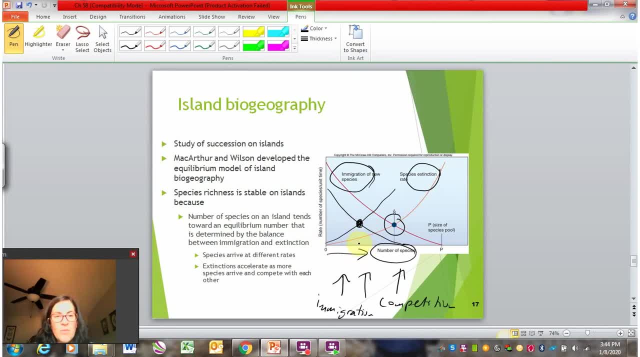 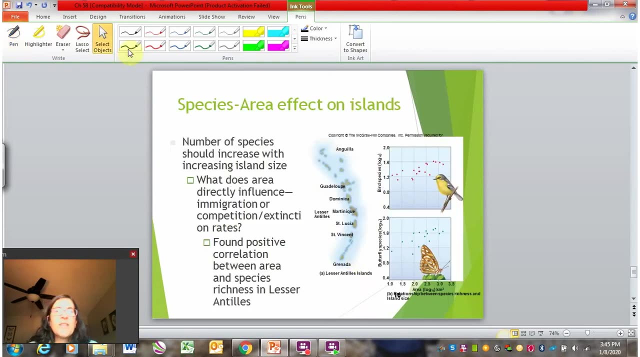 so, to recap, islands have a stable number of species because there's a balancing act between newly arriving species from the mainland and competition increasing and causing extinction within the island itself. So this idea of immigration to an island and competition leading to extinction explains why we see certain relationships between species richness on islands and 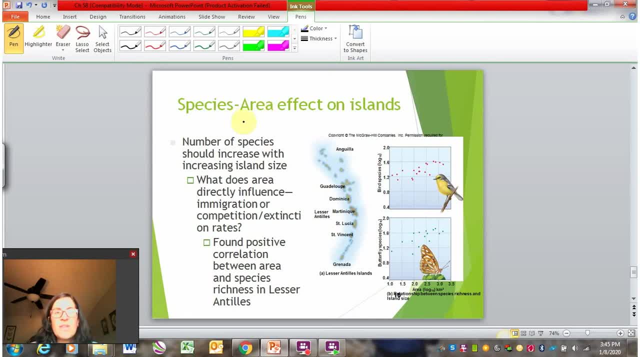 things like that. So this idea of immigration to an island and competition leading to extinction is like how big the islands are. So this is what's called the species area effect on islands, And it says the number of species should increase with increasing island size. So area. 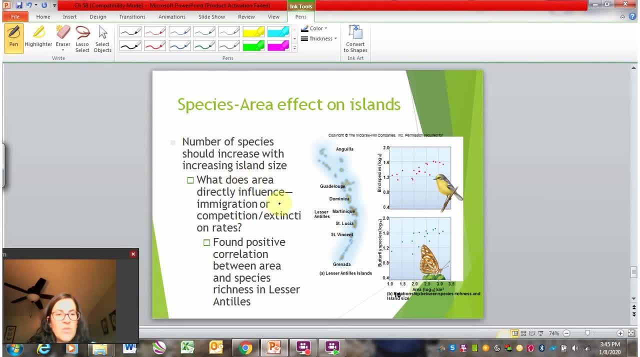 when we think about an island, what does the area directly influence? as relates to island biogeography, It affects the resource amounts. So more area equals more resources. Therefore, slightly less competition, right? So the impact of competition and extinction is reduced when you have more resources. So, again, that's why you 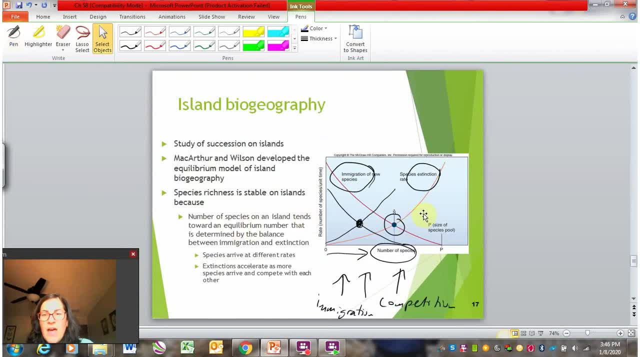 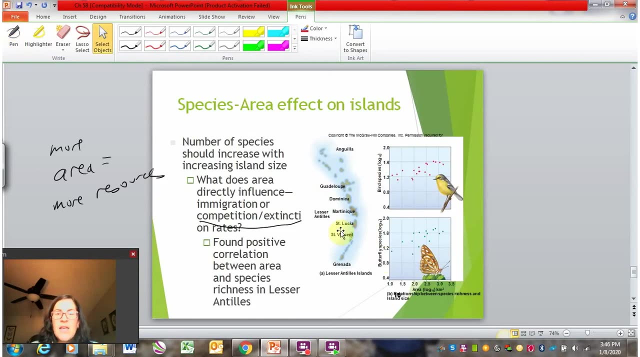 would expect that the balance point- so going back to this graph, the balance point of extinction rates would be higher over this direction. So the line might look more like this for extinction rates allowing for a higher number because there's more resources on the island And, in fact, 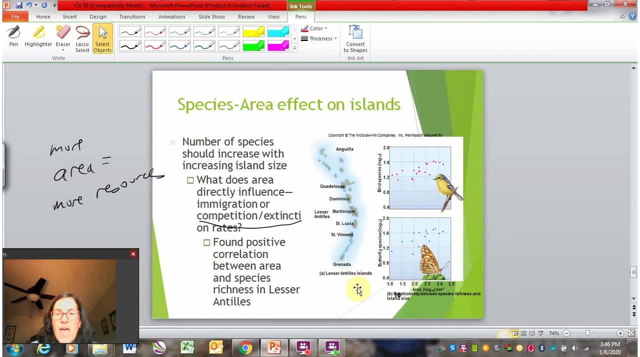 they found this to be true. So this is some data from the Antilles, the lesser Antilles islands, where you can see there's an island chain with different sized islands, And they found that the bigger the island was, the more species richness there was The island biogeography model also. 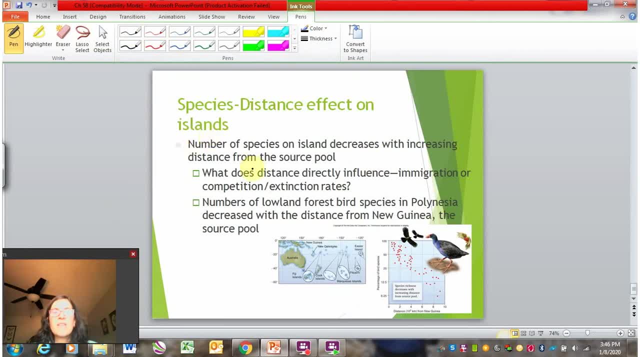 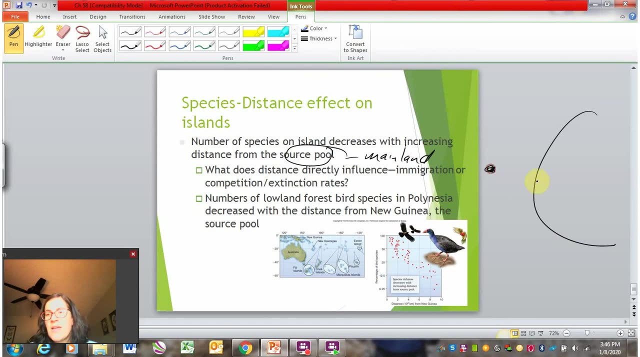 predicts a species distance effect on islands, And so what they proposed was that the number of species on islands decreases with increasing distance from the source pool. So the source pool is usually the mainland, So you have some continent and then you have some island, And so organisms are coming from. the mainland and colonizing the island, And so their proposal was that it is harder for species to get to farther away islands, And so you would expect a lower number of new species on an island that's further away and therefore a decreased amount of species richness. So if you have a